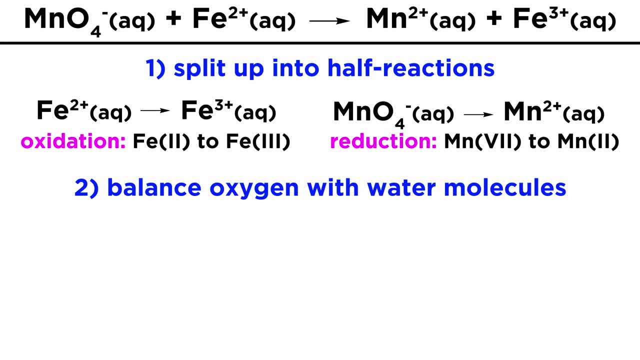 half reaction doesn't have any oxygen, so we don't have to worry about that, But the reduction half reaction does. So we have four oxygen atoms on the left because we have MnO4. So if we have four oxygen atoms, we're going to need four water molecules on the product side, because each water 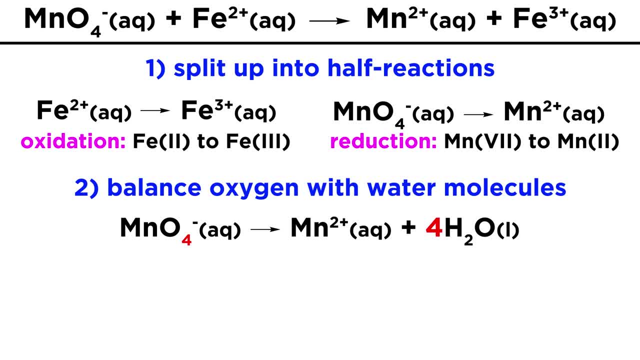 has one oxygen. So we're going to have four oxygen atoms on the left because we have MnO4- to MnO4-, So let's put four waters there Now. step three is to balance hydrogen with protons. So once again, 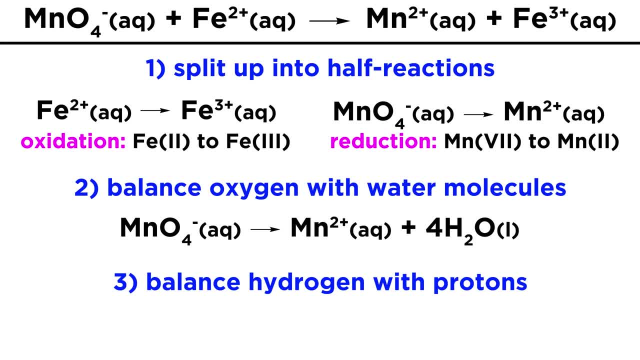 the oxidation half reaction we don't have any hydrogen, We don't have to worry about it. But we have just put four waters for the reduction half reaction. So we're going to have to balance those hydrogens. So if we have eight hydrogens on the right- because there are two per water- 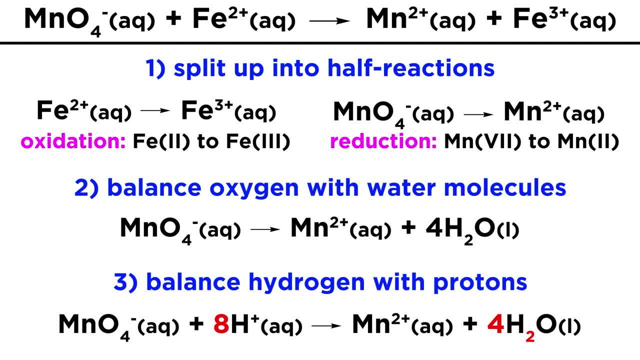 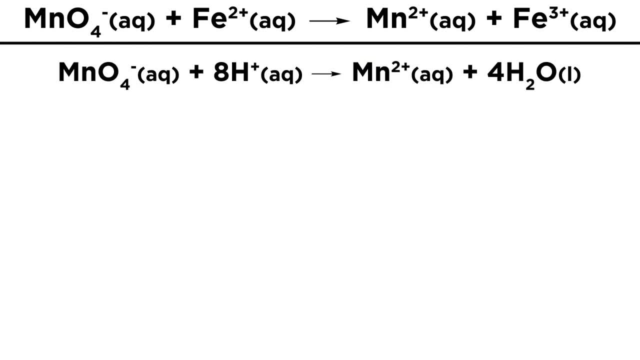 molecule and there are four waters. we need eight H-plus ions on the left. So that's the end of step three. Let's bring this back to the first step. So we're going to have four hydrogen atoms on the left. Let's bring this up to the top so we have some more room to finish up. Now step four: we're. 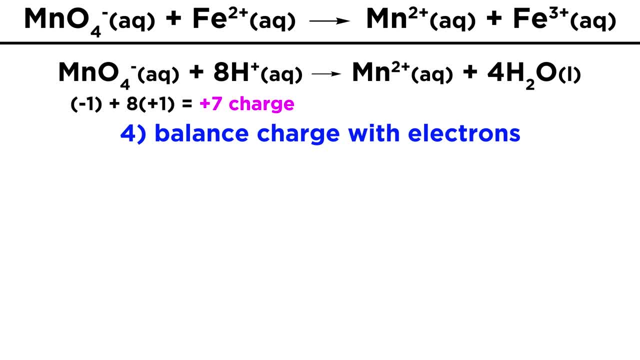 going to have to balance charge with electrons. So on the left we have a plus seven charge total because we have a minus one charge, And then we have eight plus one charges because we have eight protons. So minus one plus eight is plus seven, And on the right we just have a plus two charge. 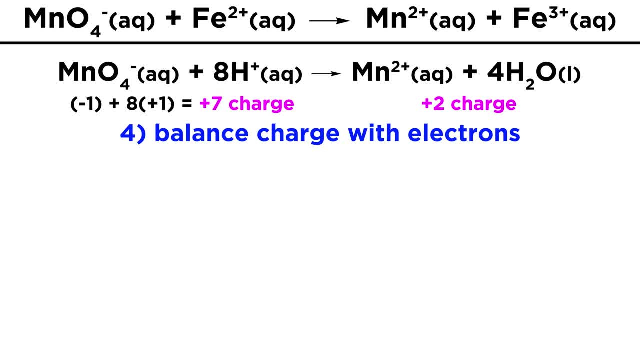 from that one Mn2-plus ion. So we have plus seven on the left and we have plus two on the right. That means we're going to need five electrons on the left to balance the charge, because if we have a plus seven charge we need five negatively charged particles to bring that. 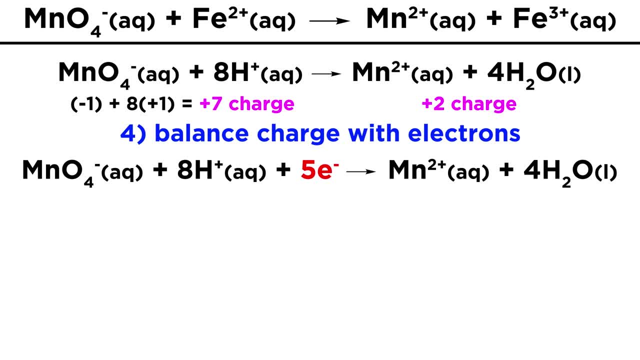 charge from seven down to two, so that we have a plus two charge on both sides. Now, at this step we're finally going to have to bring back the oxidation half reaction, because that charge is unbalanced, And so we're going to need one electron on the right to bring the three plus charge. 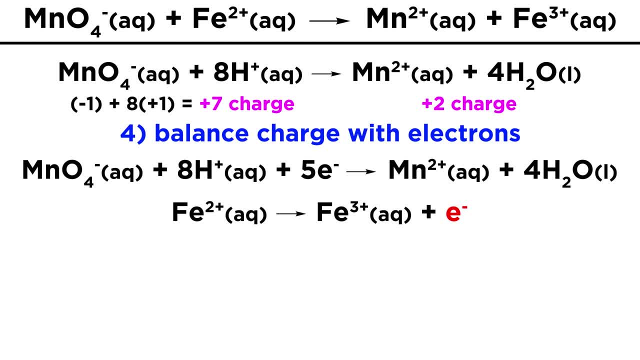 down to two plus, so that we have two plus on both sides. Now the next step is to match the number of electrons and then combine the half reactions. So we need the number of electrons in these two half reactions to be the same so that we can combine them, And on the top we have five.